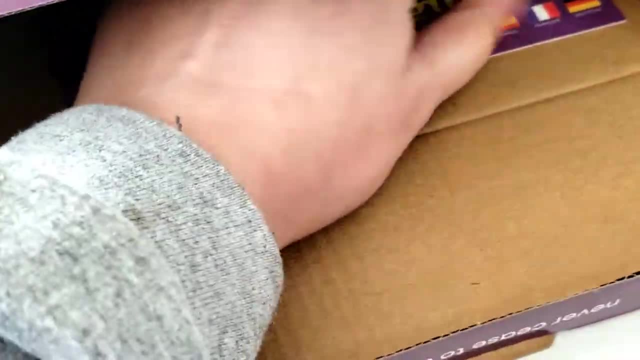 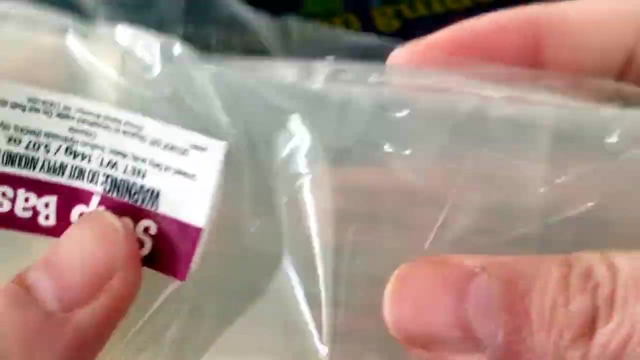 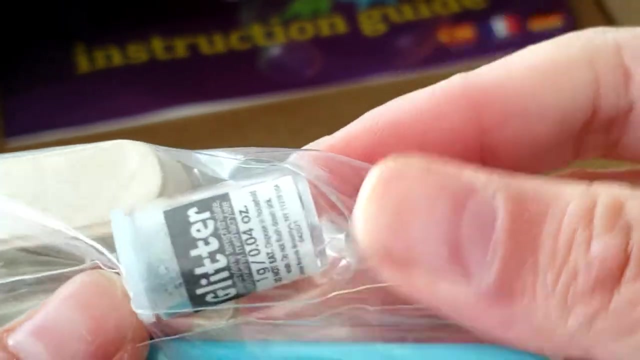 citrus scent, citric acid scent. Let's just pull everything out. Oh, here are the bars of soap. We get two chunks of soap. We get popsicle sticks, and I don't know what this little thing is. What does it say? 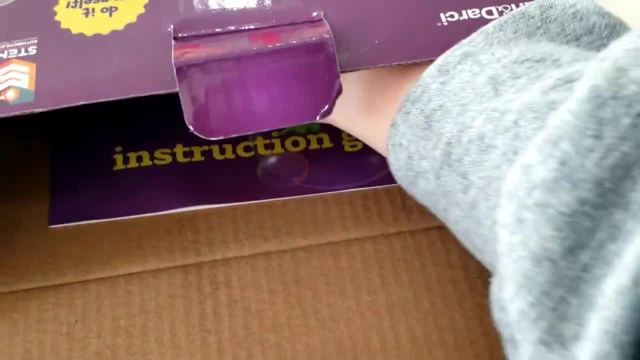 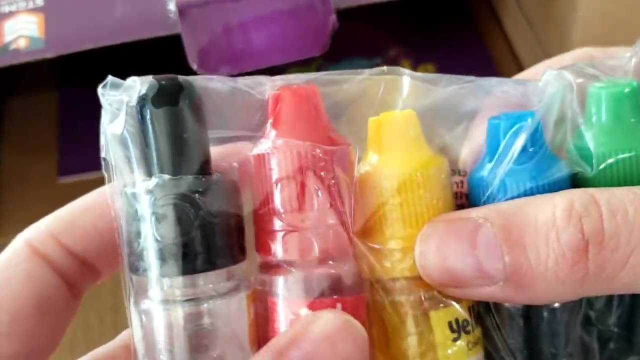 Glitter. okay, I hope it's biodegradable. And here are the cups. And here are the colors: One, two, three, four, five, six. Are these sets? These may be sets. No, these are colors. 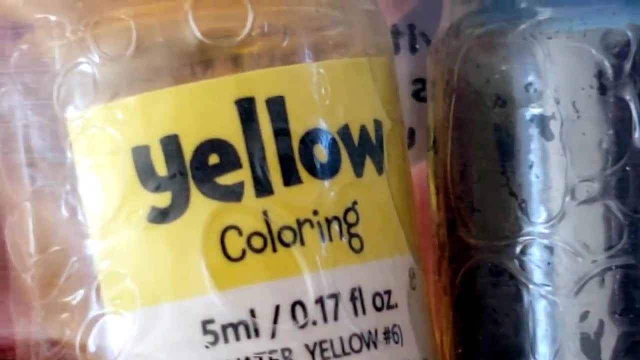 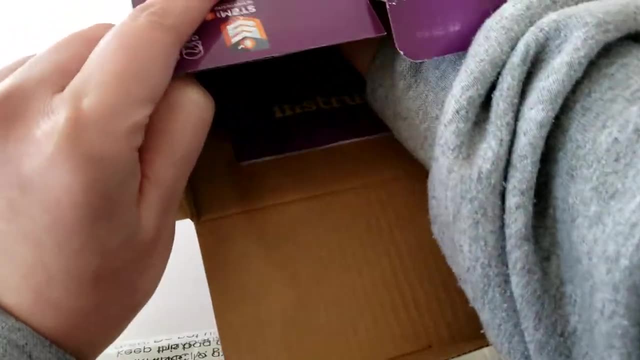 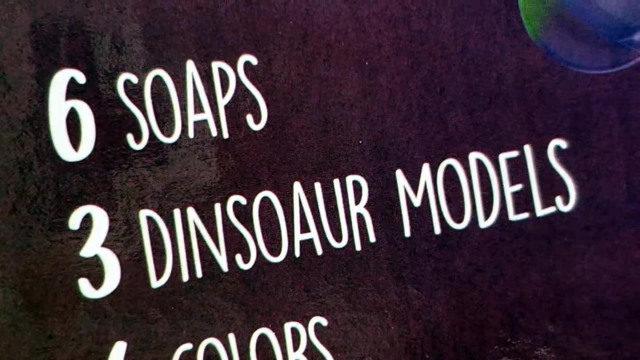 I thought it said there are only four scents, Four colors. There seem to be a lot more than that. Alright, Right, Didn't it say four colors? Yeah, it said four colors, Six soaps, Three dinosaur molds. Okay, so it does come with four colors and it comes with two scents. 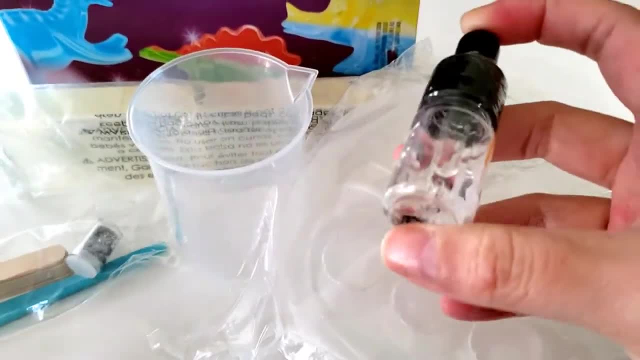 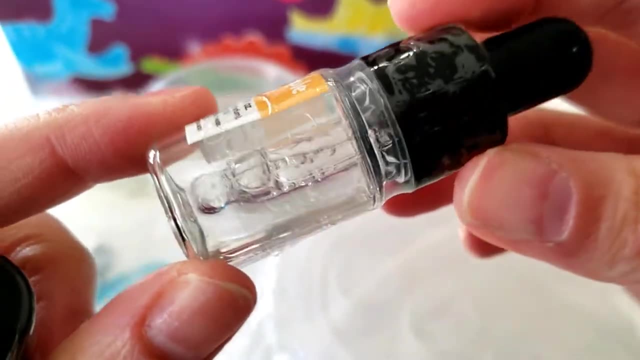 We have a green apple and a lemon, and they smell Whoa, Whoa, Oops, They smell really good. It doesn't feel like there's much in here, though. Is there even anything in here, baby? No, These are the four food colorings. 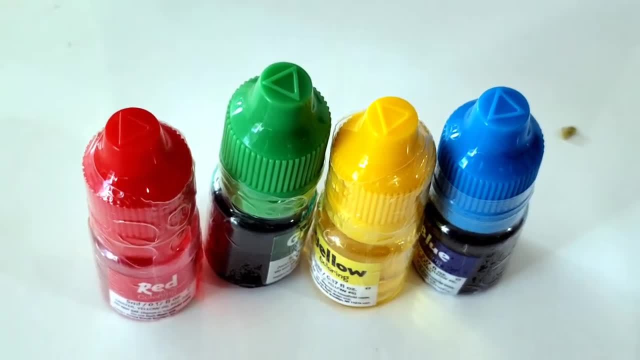 What colors were they again? Okay, I forgot to mention it comes with this pamphlet of instructions, So let me read this and we'll get started. Okay, This is the food coloring. Okay, This is the food coloring, Okay. 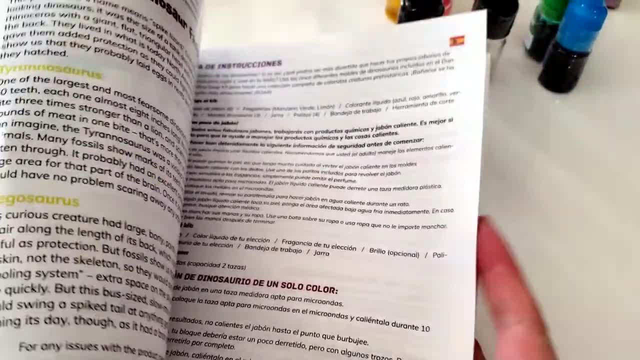 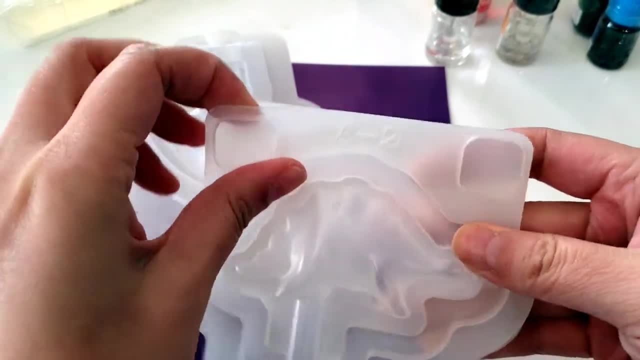 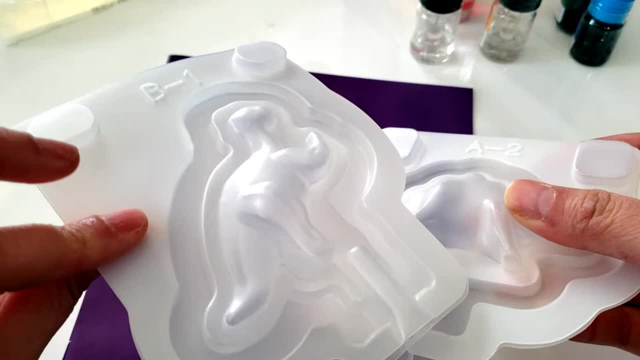 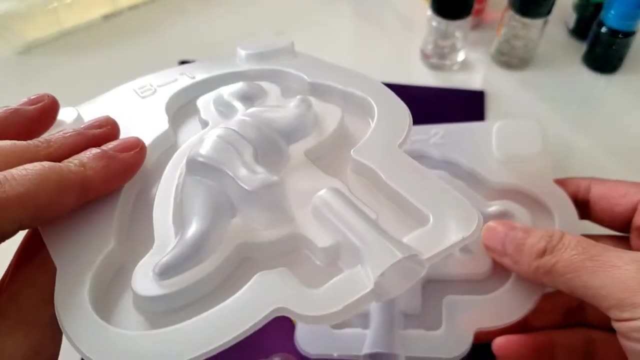 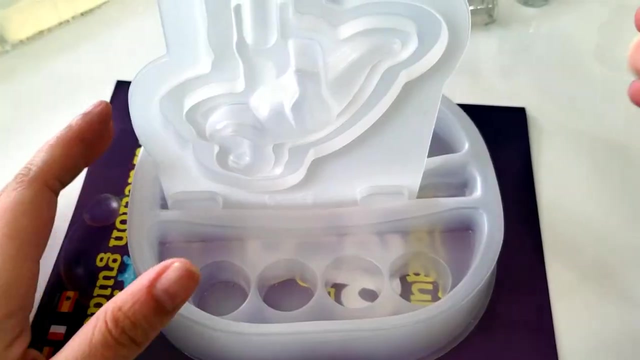 Like this would be good for a bath bomb. I think I would use these for bath bombs, But how do you pour hot soap in both sides and then squeeze it together without it spilling everywhere? maybe I should read the directions first. 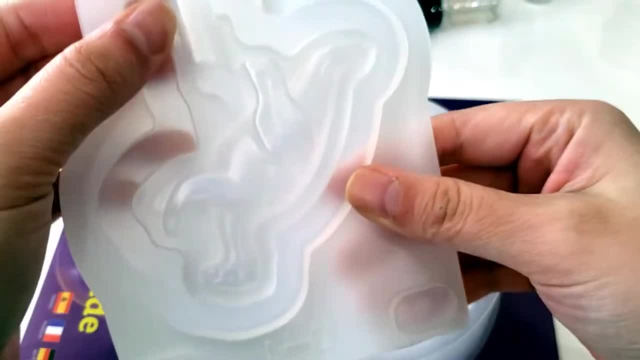 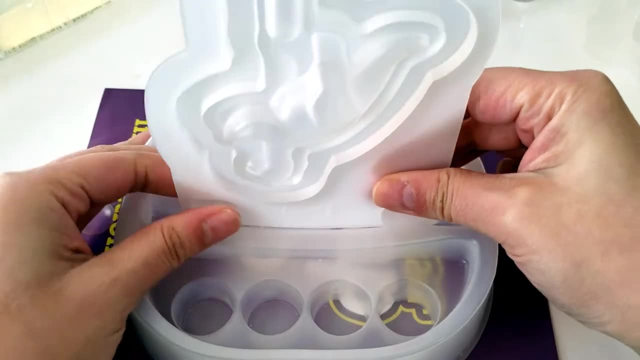 Oh, okay, So it comes with this tray. This is called the working tray. These are the dinosaur molds- is like a little pour spout here. so you have to do make sure these are closed tight and you stick this into this slot. here it says: and where's the beaker? 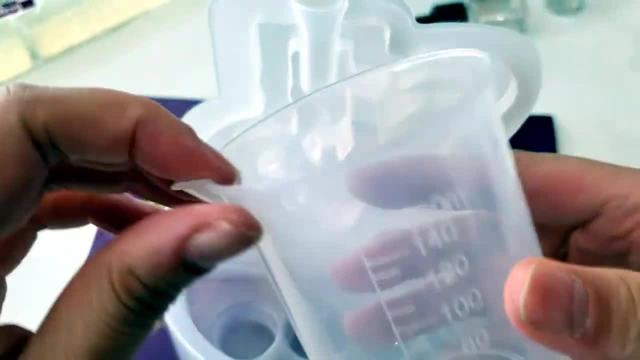 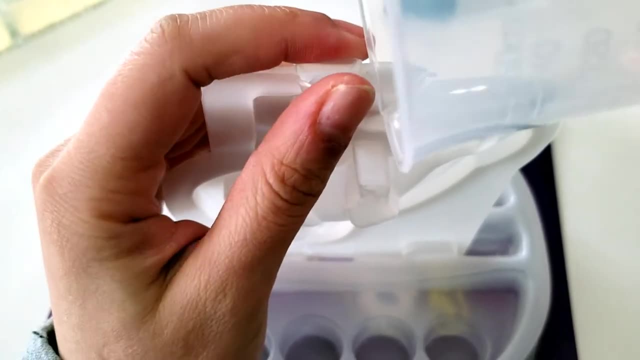 here's the beaker. so here is a beaker. you're supposed to melt the soap in your own container- microwave safe container- and then pour it into the beaker and then pour it into here. so you melt it for 10 seconds and then you mix your 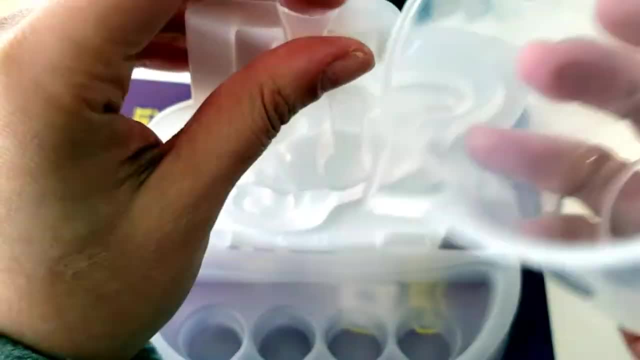 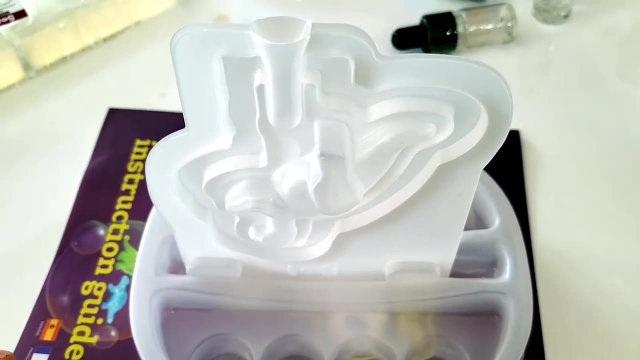 colors and glitter or fragrances in here, then you pour it in here. that's basically the gist. I'm gonna test this out and see the work. so here is the block of soap, and each block is actually cut in three pieces, so I guess that's why they. 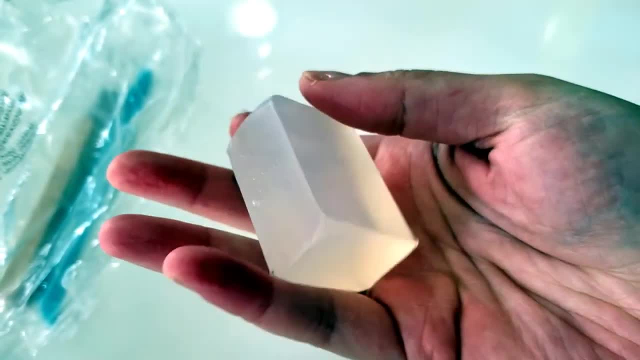 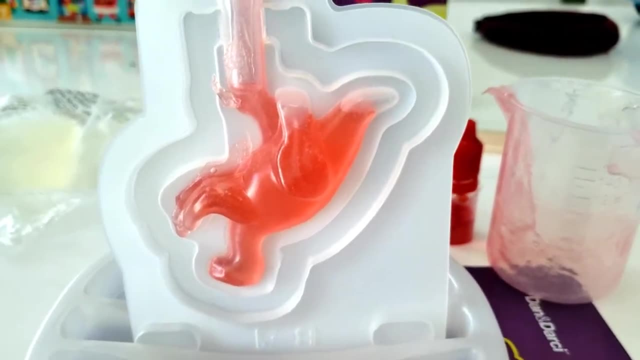 said you can make six dinosaurs. you just break it off and you melt this little chunk in the microwave for 10 seconds. this is our first dinosaur soap. sorry guys, I didn't show you the whole process because it was like very time-saving. you can see, it's very easy to make and it's very easy to make and it's very 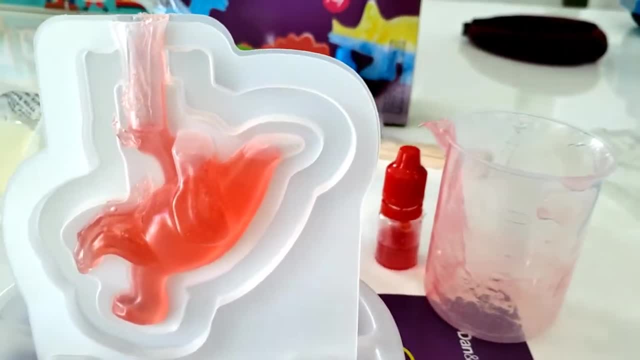 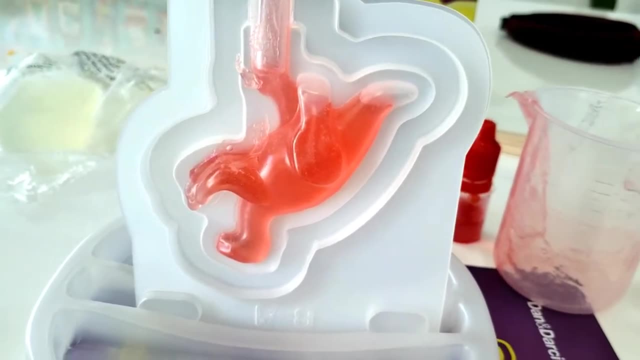 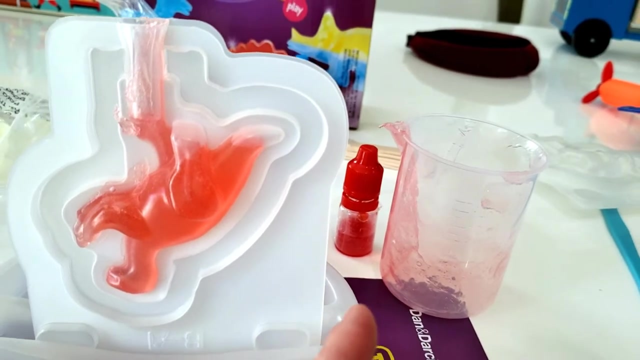 sensitive. and then this: I wanted to participate as well, so basically we added red coloring, soap coloring and the apples- was it green apple smell and he mixed it himself, so I had to be very attentive and not film. but yeah, I really simple: microwave for 10 seconds, add the coloring, mix, mix. 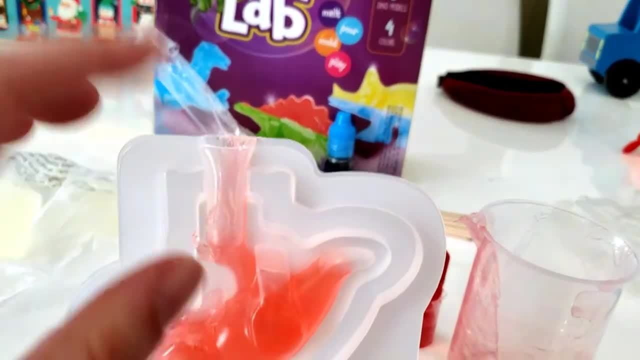 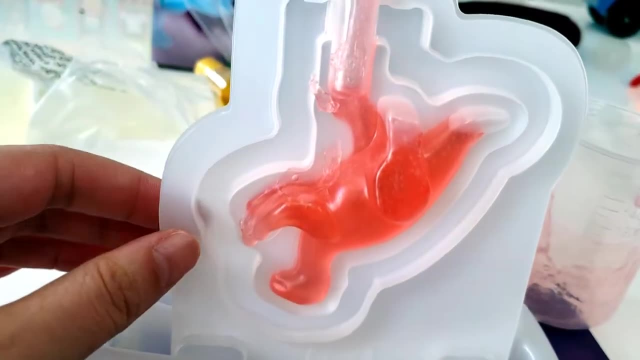 mix, add the smell mix, mix, mix and then pour it into the spout. in here this tray thing is a little bit flimsy. like this, mold will tend to want to pop out, so you're gonna want to use one hand to stabilize it and then pour it in. hopefully I can film the process for the next one, but right now 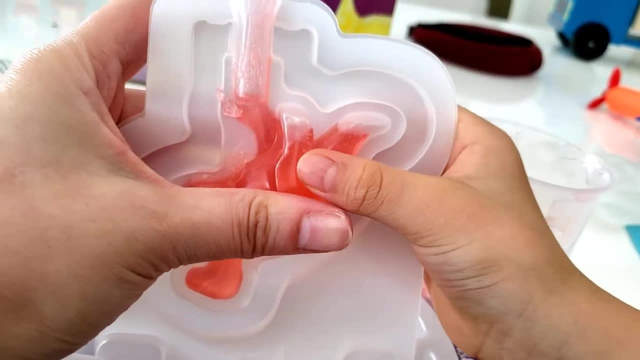 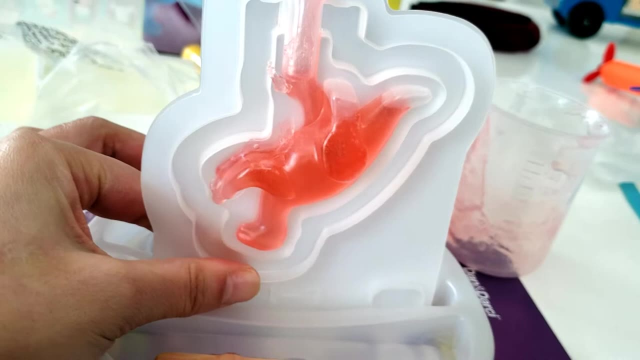 I'm just letting this one cool. and, yeah, it's warm still, so you're gonna wait for it to be totally cold, okay, and hopefully hold it centered in place. it's a lot smaller of a soap than I thought. you know what kind of dinosaur this is. 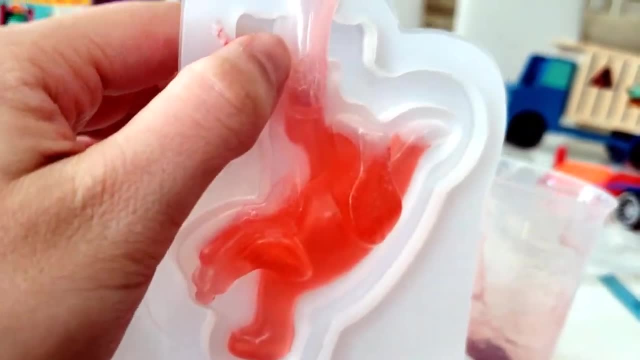 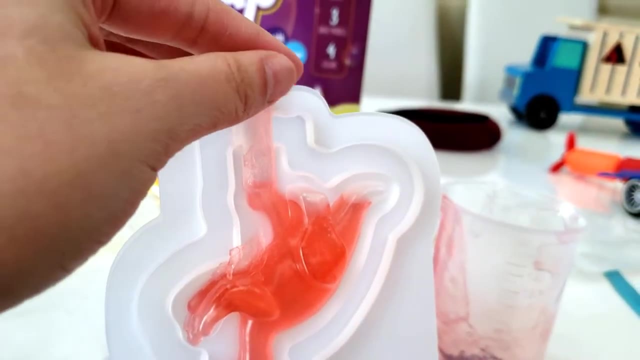 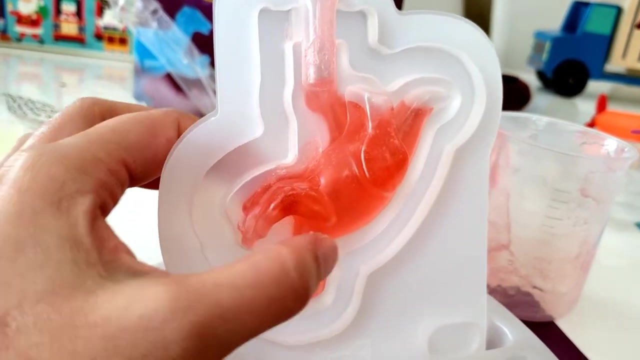 I don't even know if it filled it all the way up. I can't tell. oh, it's a t-rex, are you sure? I can't tell. anyways, yep, pretty cool, though can definitely reuse these to make little mini bath bombs in the future. I do want. 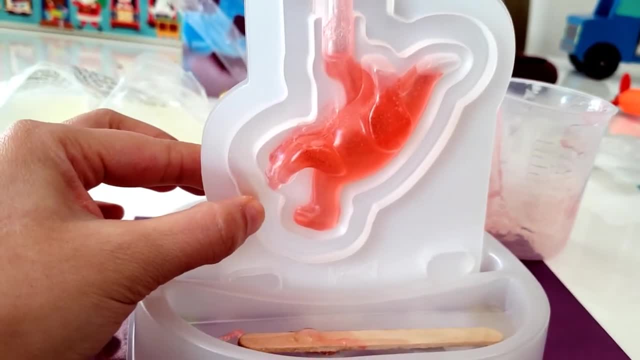 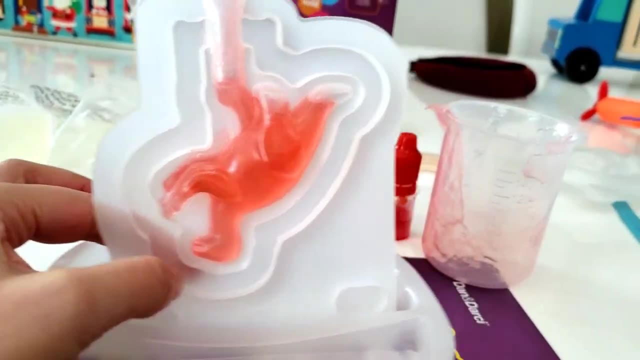 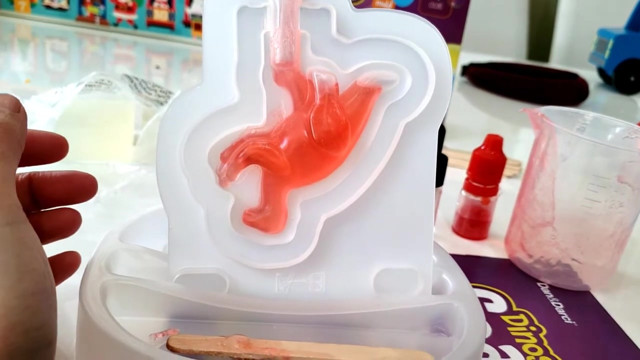 to make bath bombs. if you want to see us make bath bombs, make sure to thumbs up subscribe. leave a comment down below. but yeah, overall this kit is a decent. the food coloring gave us quite a hard time because even after you open it like nothing came out and it's too hard for the kids to squeeze themselves and he. 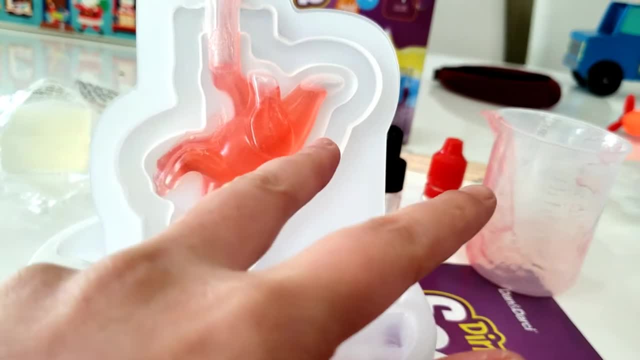 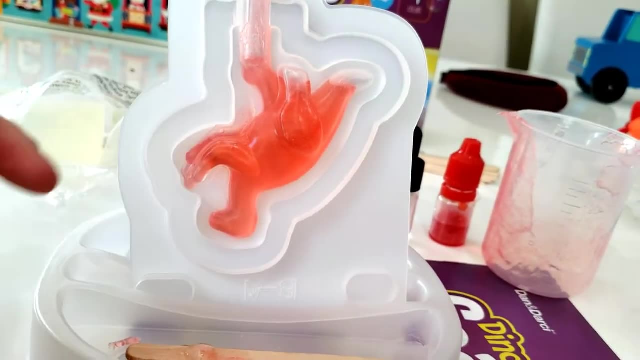 really wanted to put the food coloring in himself, and I even had to cut off, like the tip of the food coloring to even let myself be able to squeeze it out. and it's still really, really hard. I'm using all my strength just to squeeze out one. 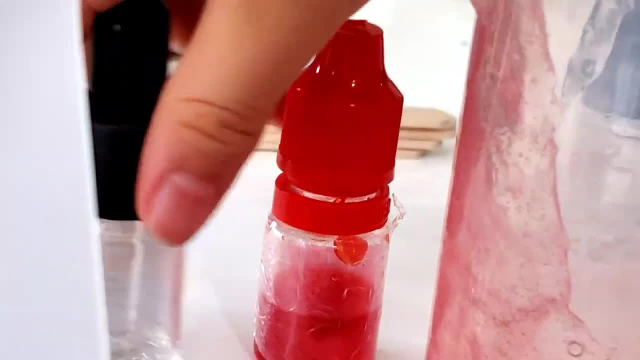 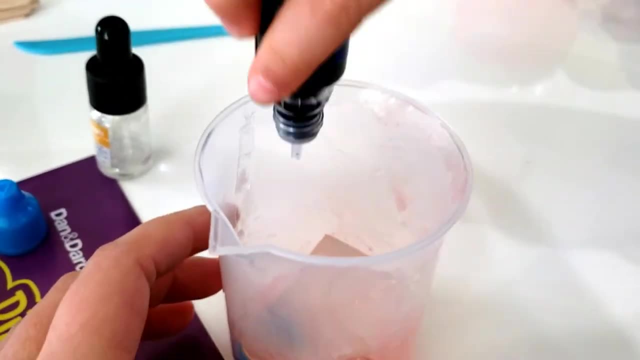 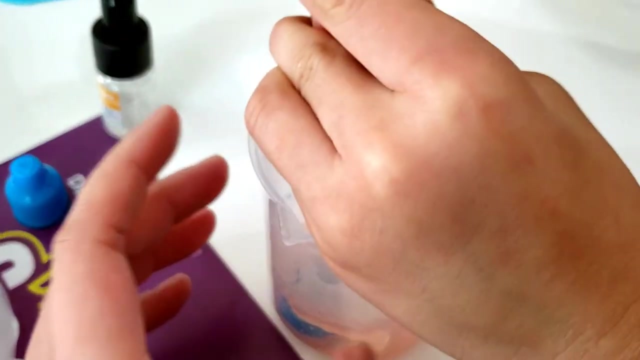 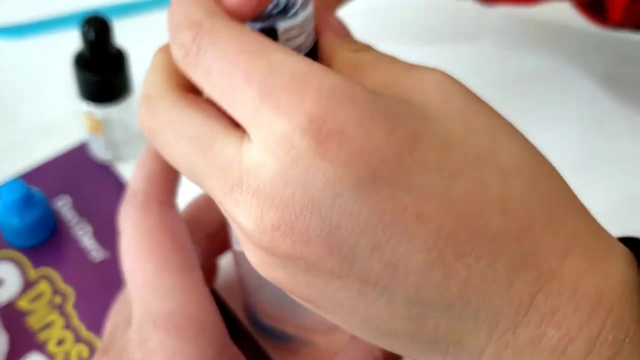 drop. so yeah, that's annoying, this thing right here, very annoying. but yeah, that's all you can add the color. make sure it goes into the cup. please don't shake it. squeeze it um. is it working? is it working, baby? yeah, okay, okay, stop, let me see how much you. 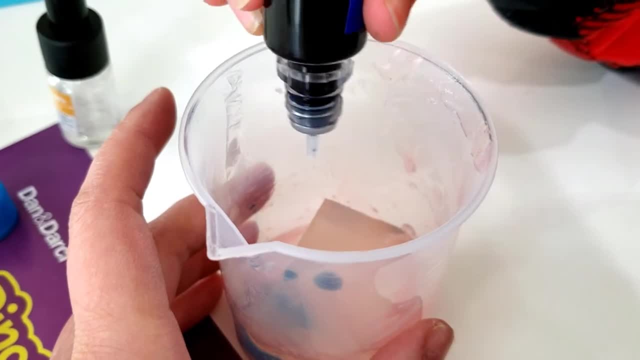 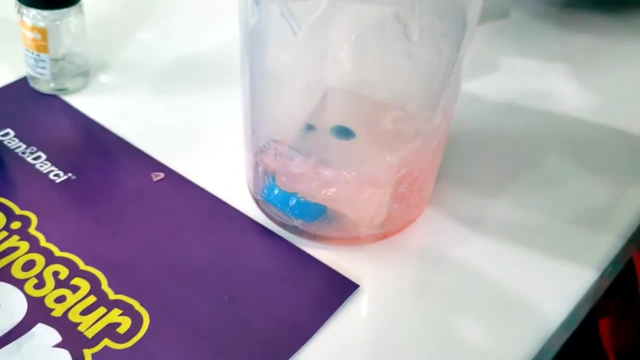 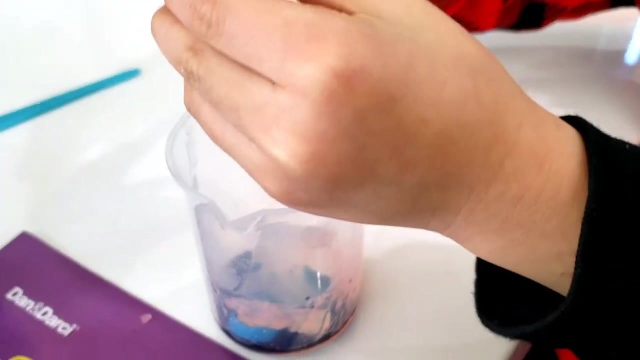 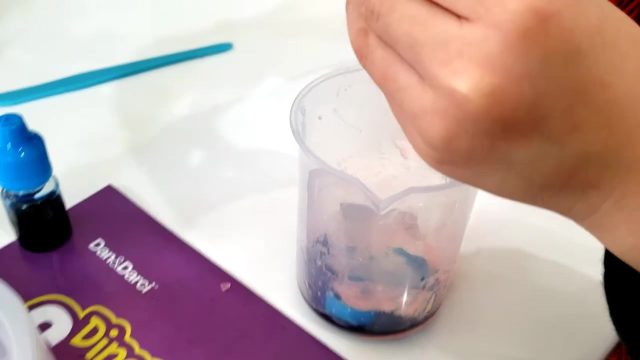 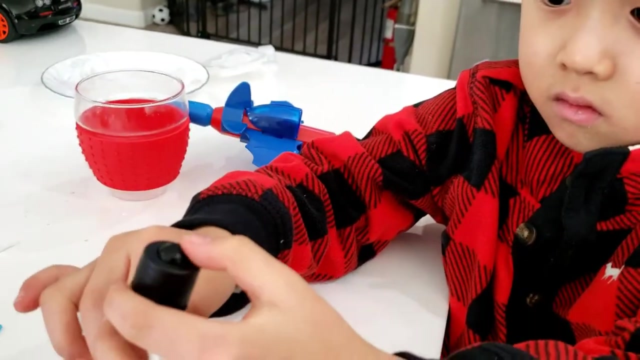 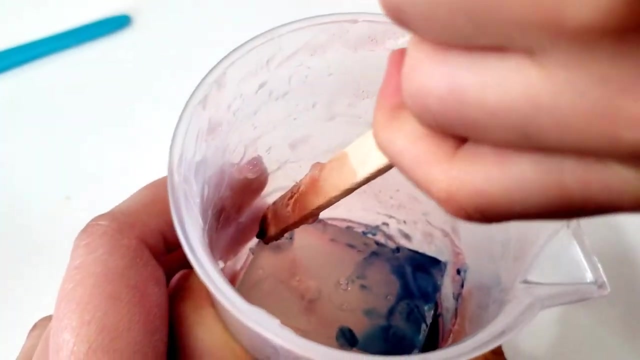 added. okay, go add our scent. what scent is this baby? what scent is this baby? green apple, green apple, okay, okay, add your scent. now. mix it up like that. why are you mixing it like this? oh, is it hard in slow motion? oh, it hardened already, so you do have to move fast. 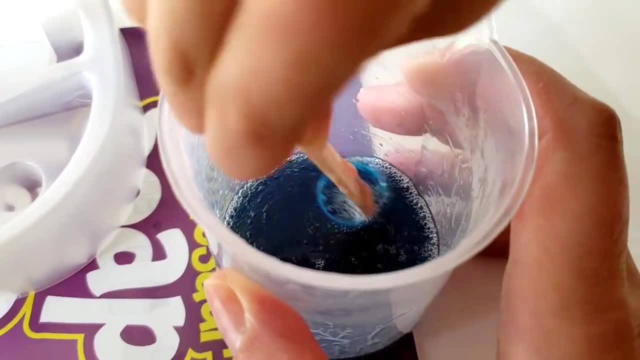 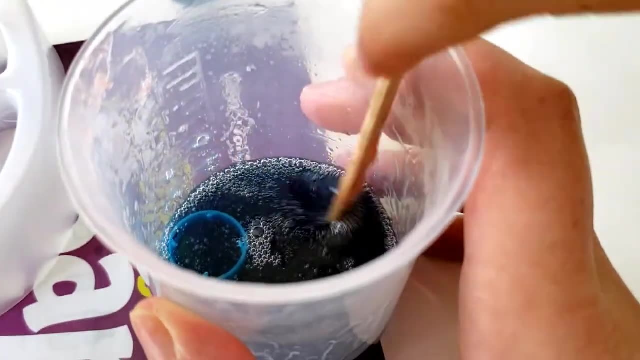 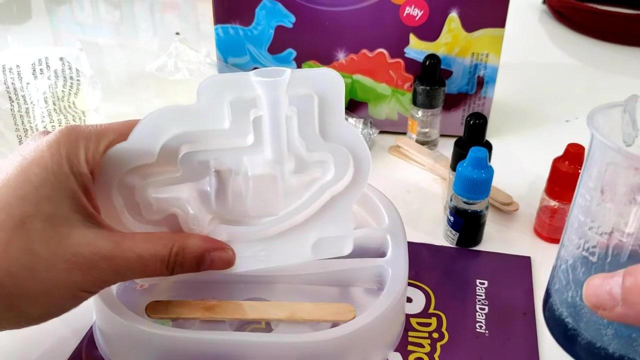 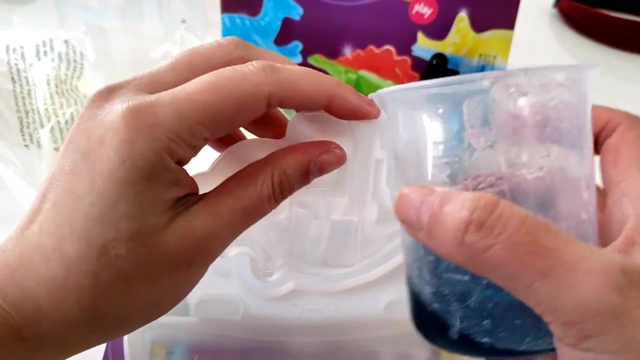 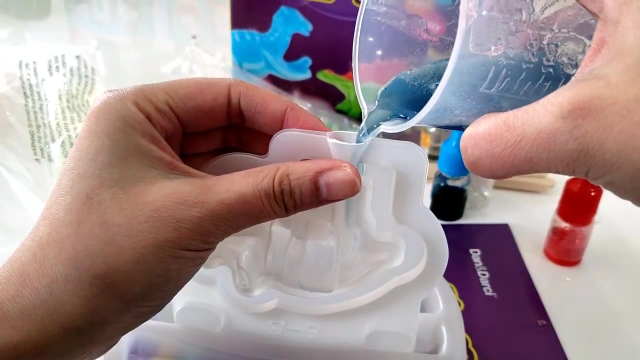 there we go: stir, stir, stir, huh. what color is it? blue, don't you think more? no, that's enough. we're gonna pour see that the base is not very sturdy, so this should definitely be done by an adult. okay, I'm gonna find the beaker right here. I'm gonna 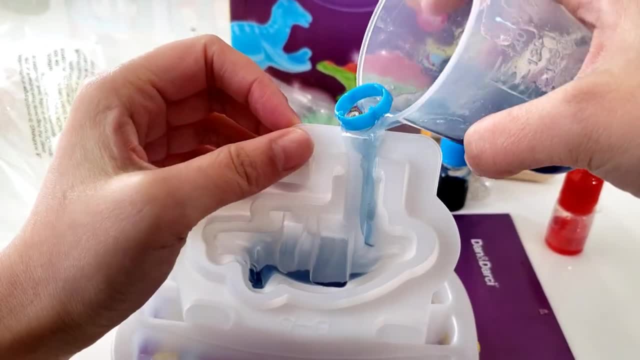 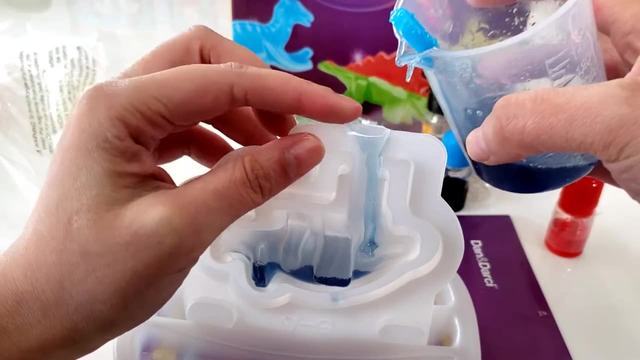 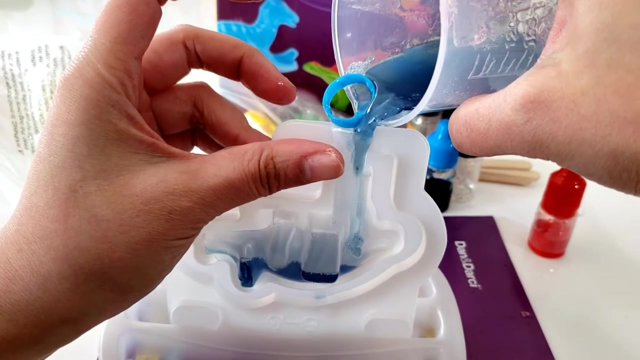 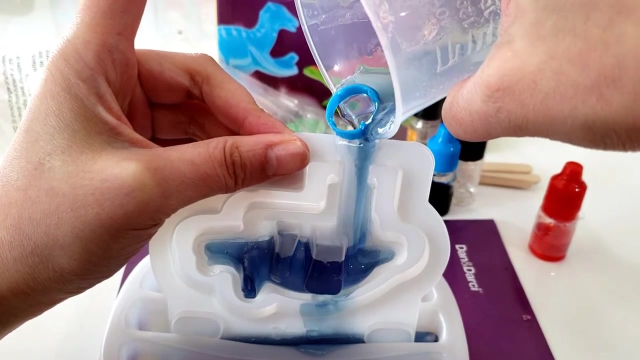 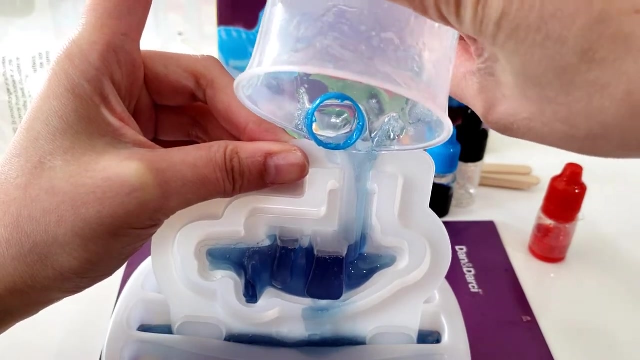 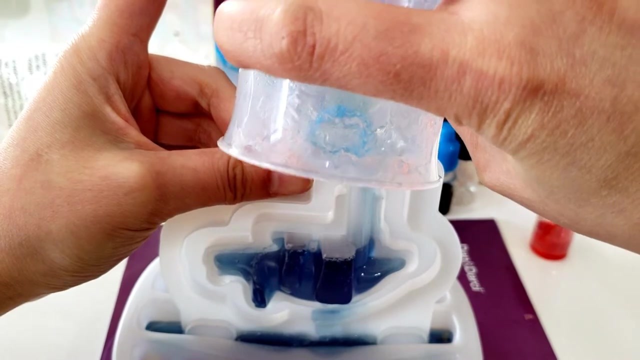 good, is it working? is it working just a little bit more? okay, hold on, find the hole. okay good, Did it fill all the way up? Yeah, Yeah, Huh, What's that? What Ugh? It's leaking A circle. 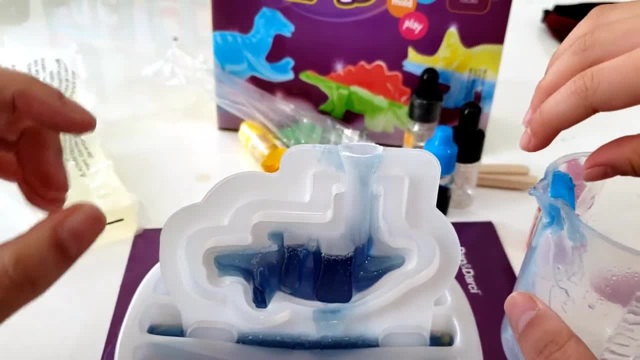 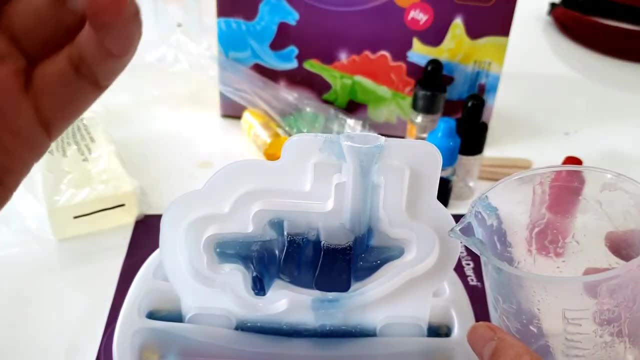 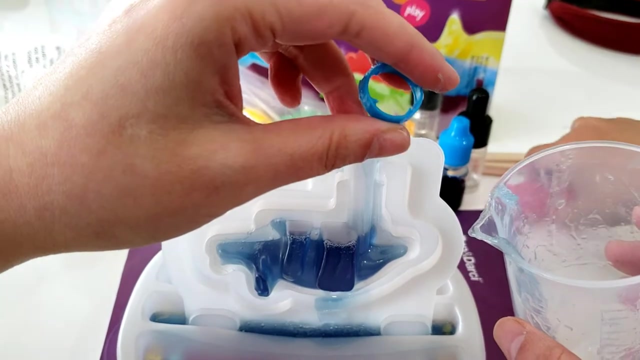 A circle There. Where, Where, Ta-da, What Here? Where'd this come from? Ugh, Where was this from? From the blue, From the top, Yeah, Of here, Yeah, Oh, It must have just hardened. 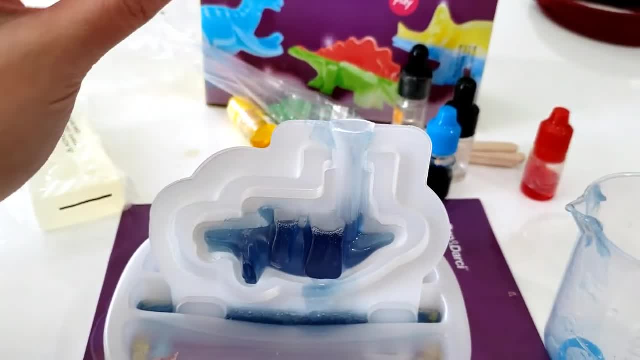 Okay, Well, we'll save that for next time. And where's the white? So there you go. And where's the white color. It mixed into the blue, Okay. so it looked like this one leaked out the bottom. Maybe it wasn't as tight as I thought. 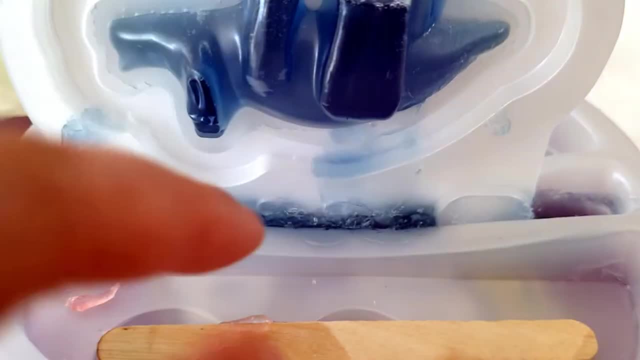 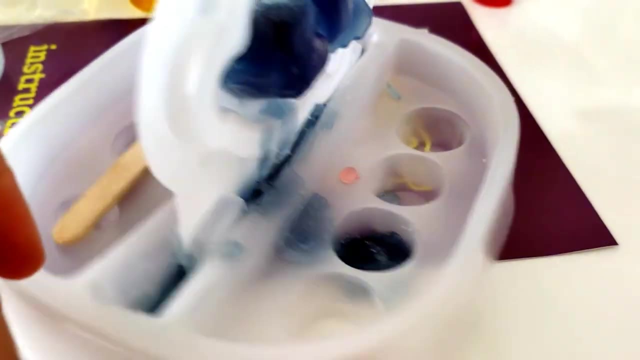 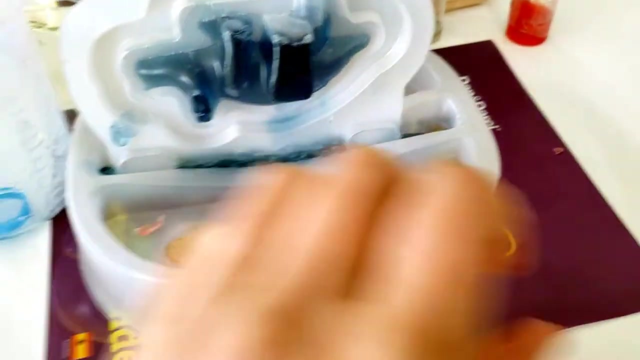 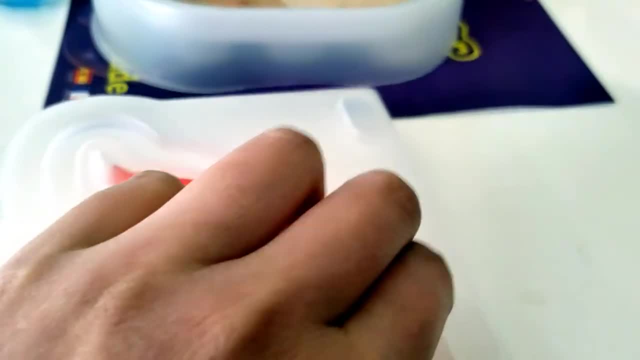 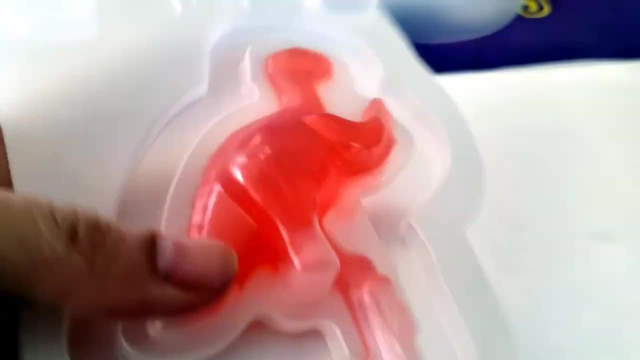 Okay, Okay, Okay, Okay, Okay, Okay, Okay. I think I was evil. Yeah, All right, so we're done with this one. We're done measuring these. And then there are some golden evens here that are like different colors. 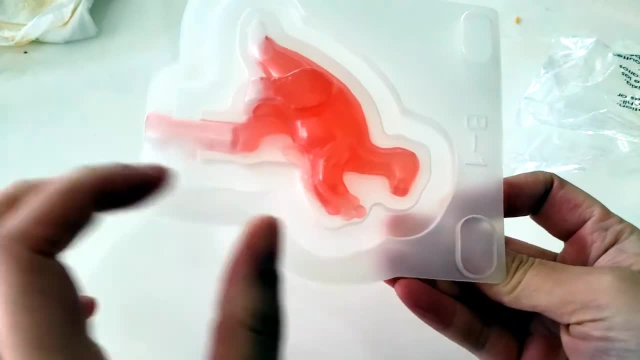 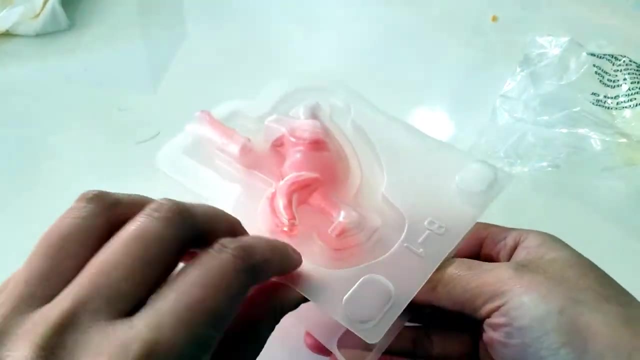 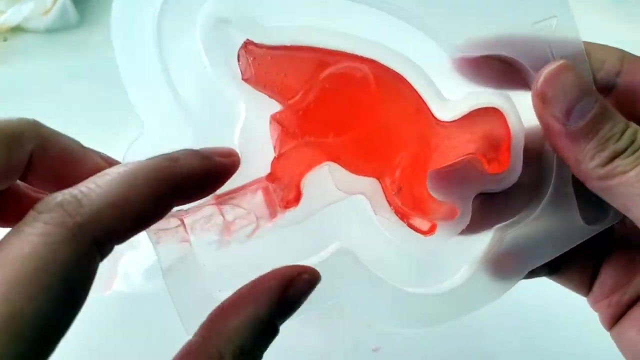 Probably because the one above is a little bit pinkish. This is a few colors that'll look different to what they look like. I still don't know what dinosaur this is. baby says it's a T-Rex. I can't tell like. 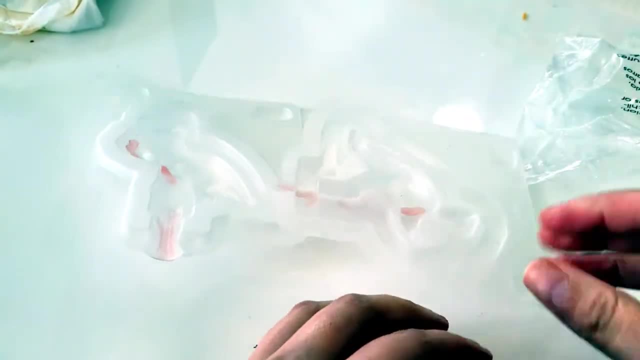 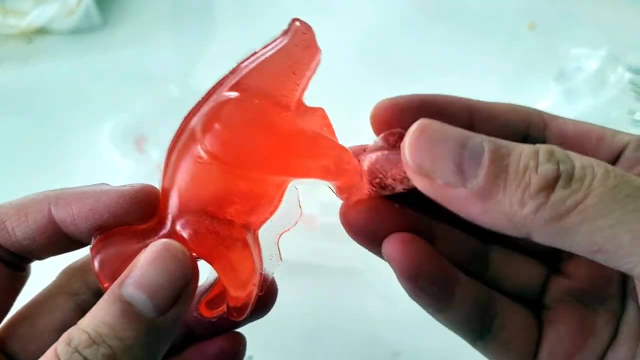 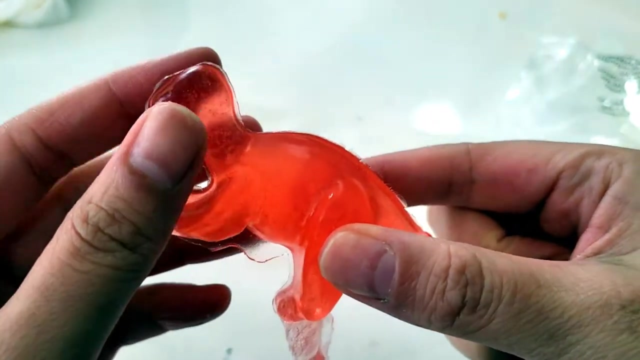 is this part part of it? okay, I guess not. it broke off. we didn't. whatever this is supposed to be, didn't fill all the way. oh, it's a dinosaur like this. oh, it is a T-Rex. 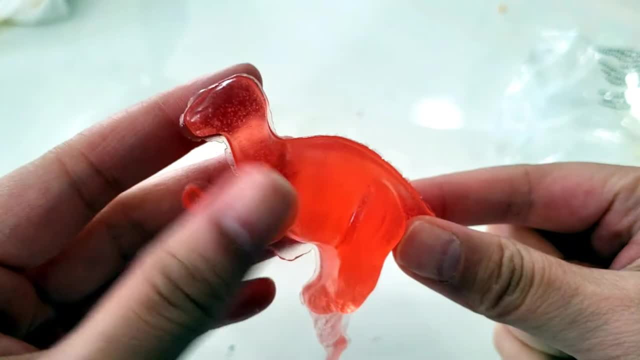 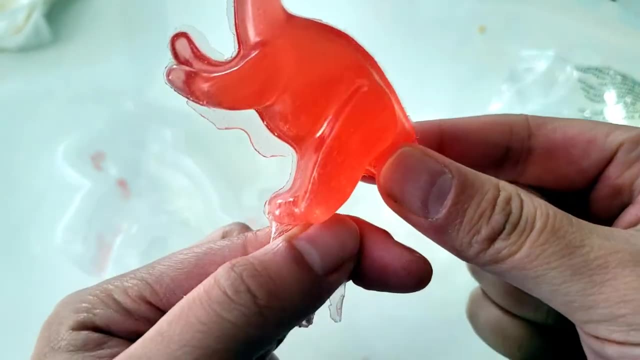 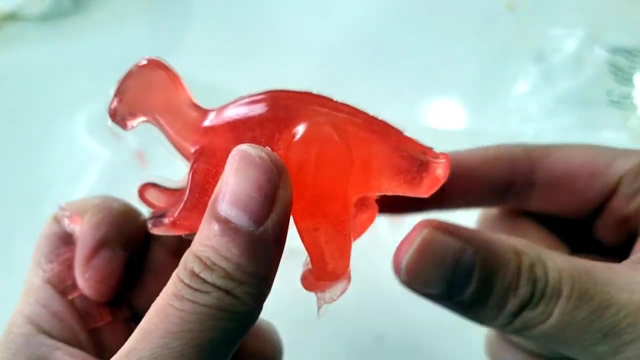 oh, but his tail is so short. some kind of dinosaur like this. unless I broke something off, unless this part is supposed to come off, I don't know, maybe baby T-Rex or baby something, I don't know.